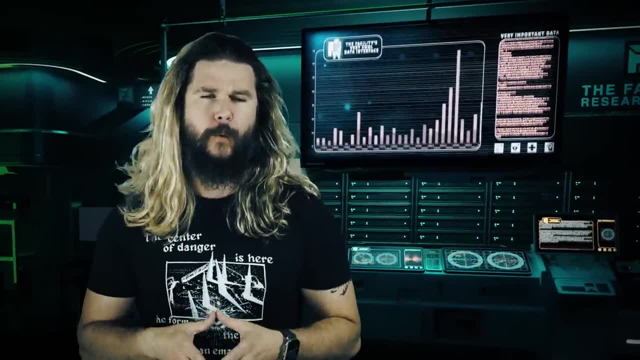 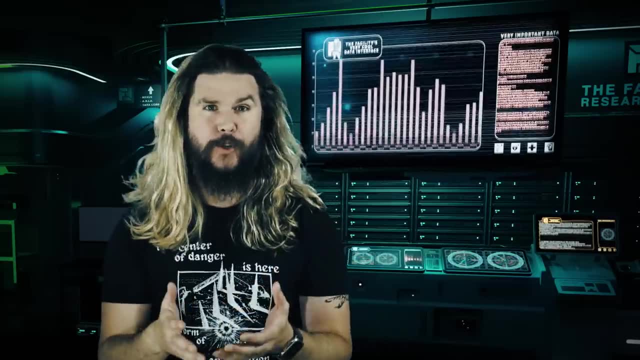 As part of the facility's nuclear education initiative. no, I won't be grading on a curve. I've tried my very best to explore and explain the pain points people have that prevent a rational evaluation of nuclear power. And if you are an iffy on nuclear power it probably has to do with. 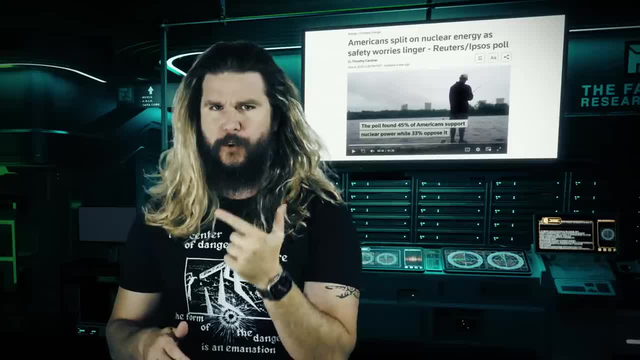 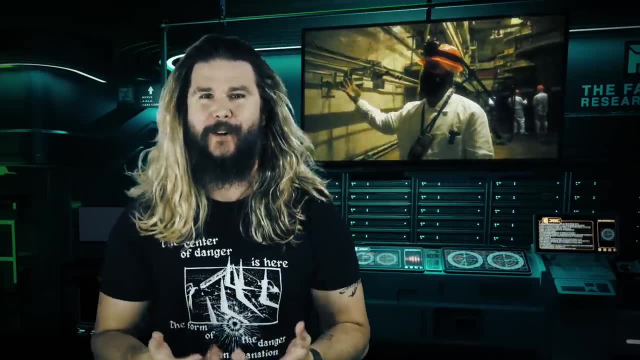 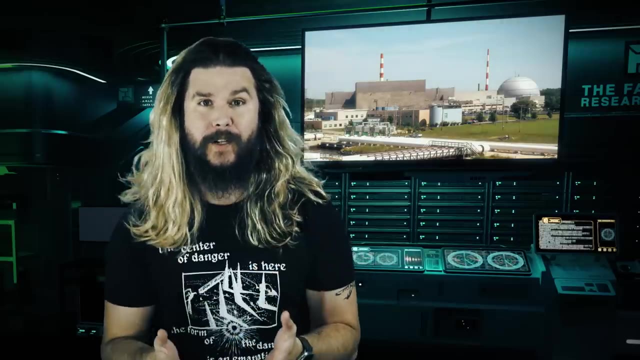 either the fear of a nuclear meltdown or what we do with nuclear waste Now. while I've been to both Fukushima and Chernobyl at this point to show you what nuclear meltdown aftermath really looks like, I've never been to a working nuclear power plant to show you what nuclear waste actually looks. 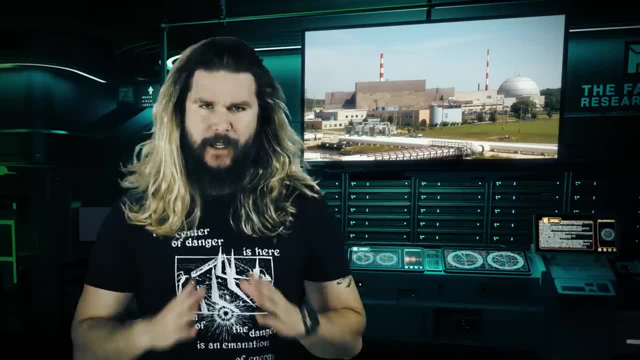 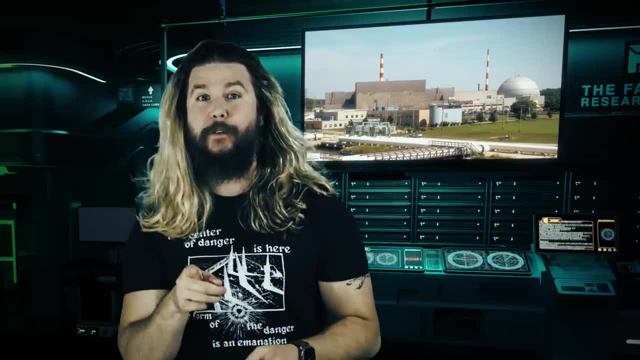 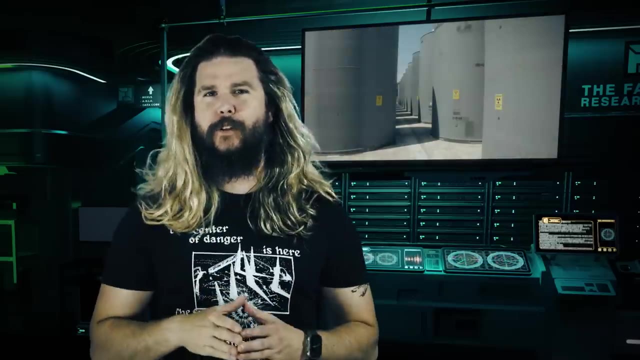 like. Well that changes today. Today I'm working directly with the United States government and the largest operator of nuclear power plants in the country to give you an up-close look at how nuclear waste is actually generated and stored. Hopefully, by the end of this video you should be. 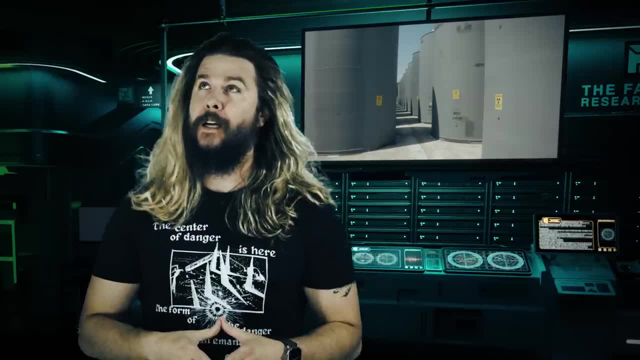 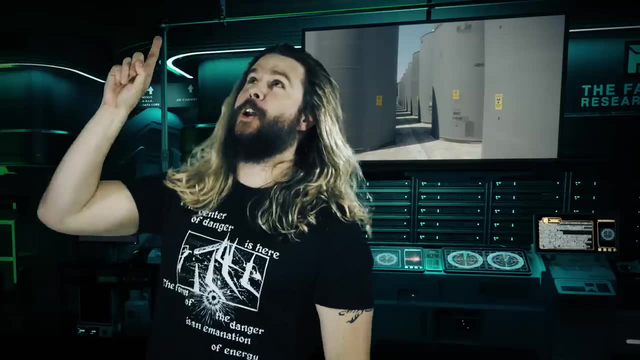 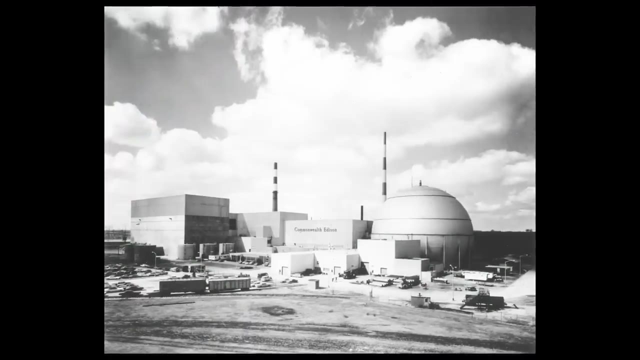 able to form an informed opinion. Aria, ready the helical ascension. Do you mean the helicopter? Yes, To Illinois, Now entering the facility. The Dresden Generating Station, which first came online in 1960, is the first privately financed. 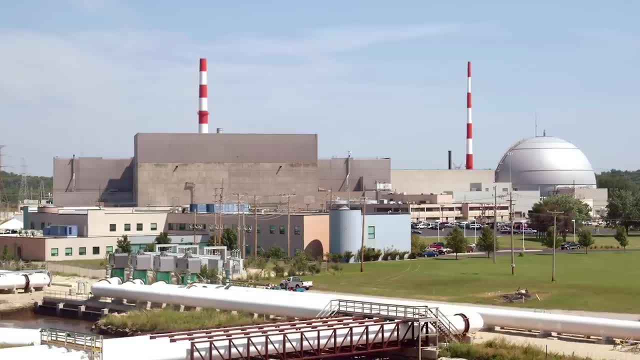 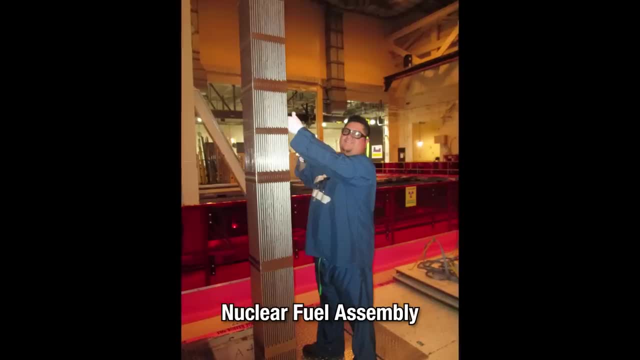 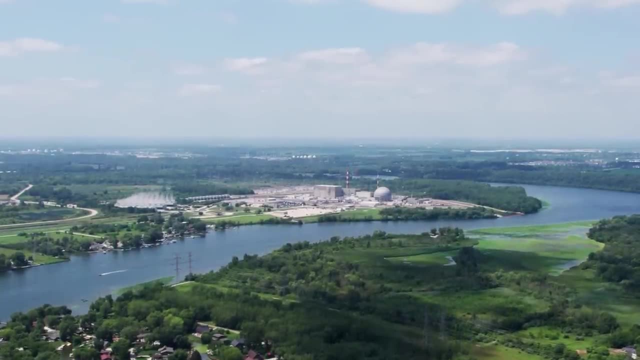 nuclear power plant built in the United States. It's owned and operated by energy company Constellation and houses two boiling water reactors that each produce enough electricity to power one million homes. Dresden turns out to be a perfect place to learn more about nuclear waste, as it is immediately northwest of the MORAS operation. 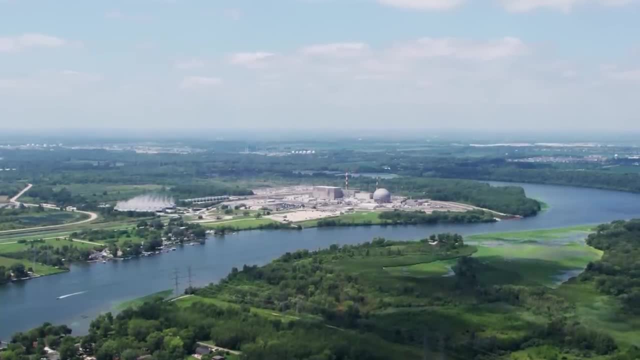 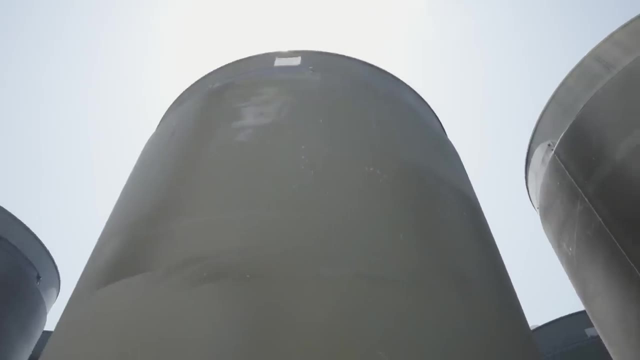 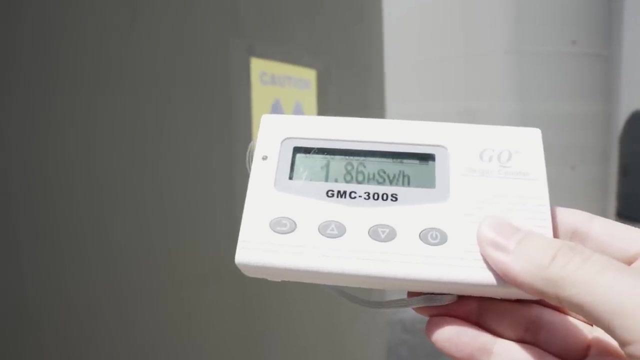 the only de facto high-level radioactive waste storage site in the United States. I visited Dresden in July of 2023. to make a simple point: Nuclear waste, despite its terrible reputation, is some of the safest energy production-related waste there is. It's 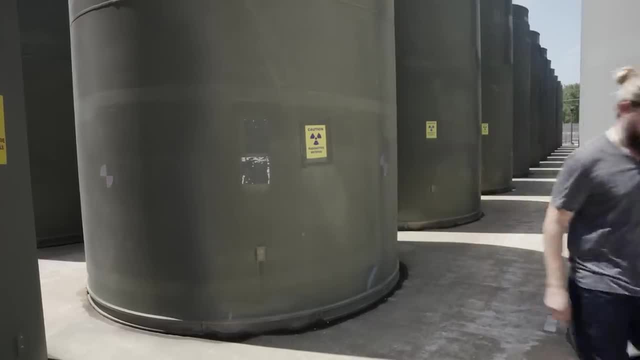 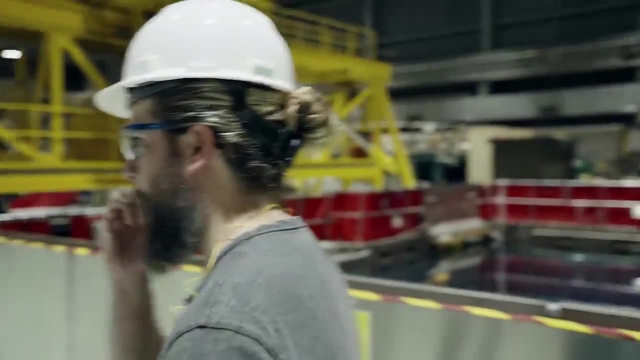 so safe, in fact, that a PR team, nuclear engineers and armed guards. let me do this. What is the point of the nuclear waste system? It's a waste that literally업. but we'll get to that later. Before I even set foot at Dresden, it was made very clear to me. 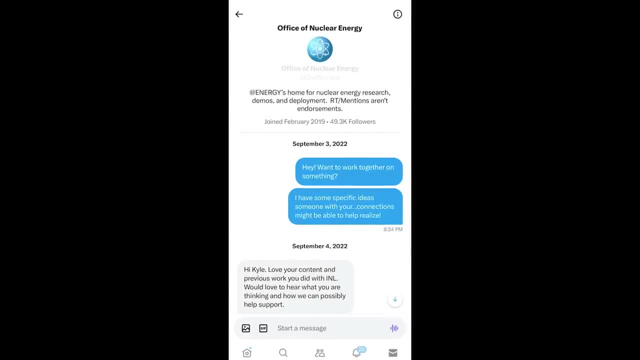 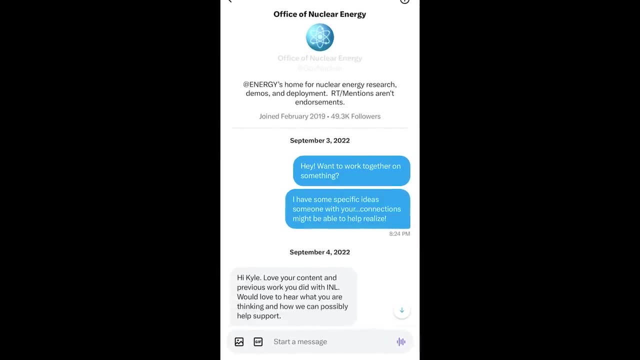 that safety was the top priority. I had to slide into the DMs of the White House's Office of Nuclear Energy and then it took 10 months of conversations to lock in a visit to Dresden. I got background checked and asked about my previous nuclear excursions to Chernobyl. 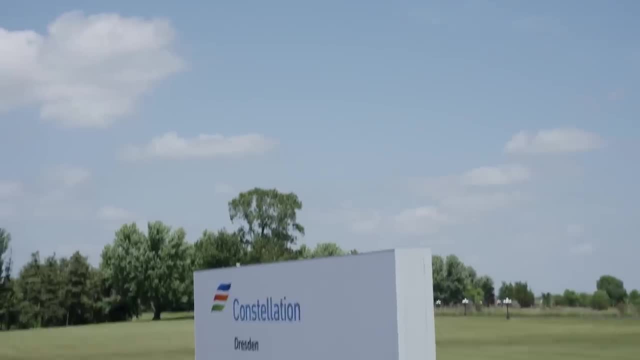 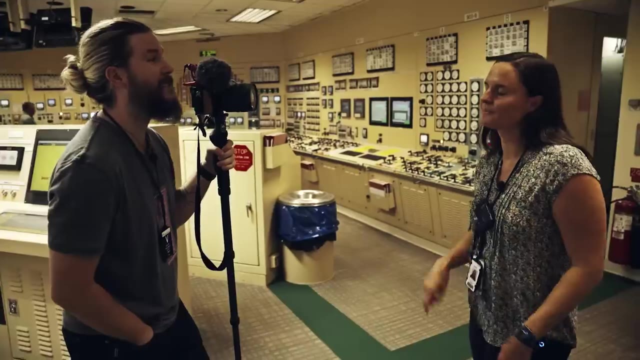 and Fukushima, as it was relevant. Once I was in Illinois, security was stepped up again. We weren't allowed to film anything remotely related to on-site security. My Kevin and I had our bodies screened and our camera lenses checked. Modern lenses are. 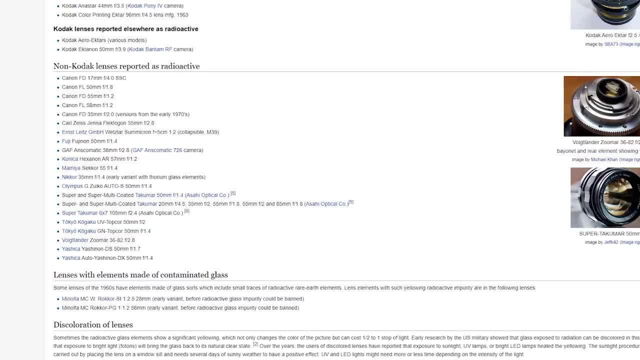 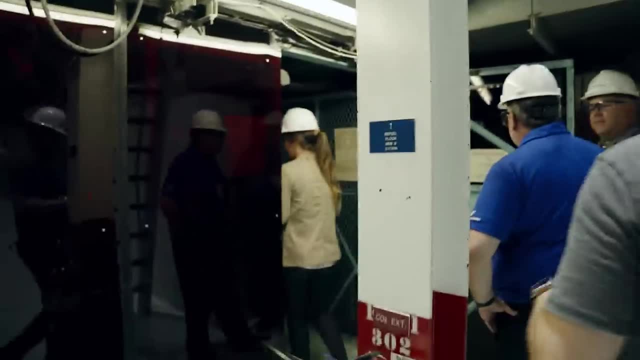 sometimes made with trace amounts of radioactive thorium which plant sensors immediately pick up. We were followed at all times by multiple escorts, including an armed guard. At the end of the trip we would have our footage screened for any frames showing security installations. 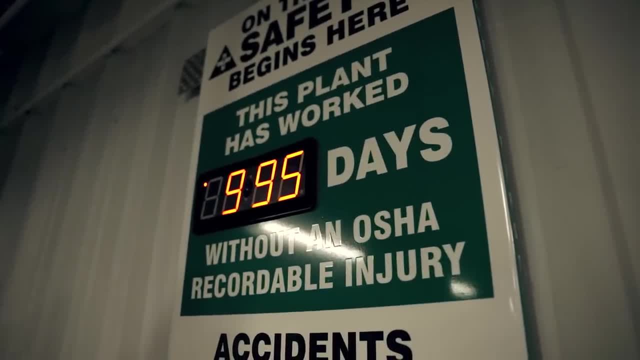 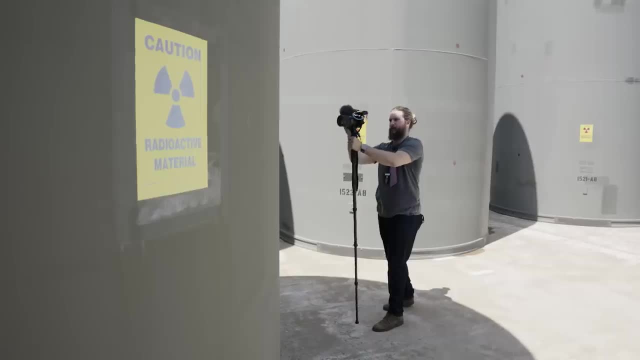 It was all much more comprehensive than what I experienced at Chernobyl and Fukushima, but that makes sense, as this power plant is in operation and those are not- Even though all of this was a little nerve-wracking- were the boots I was wearing in this video still contaminated from Fukushima? 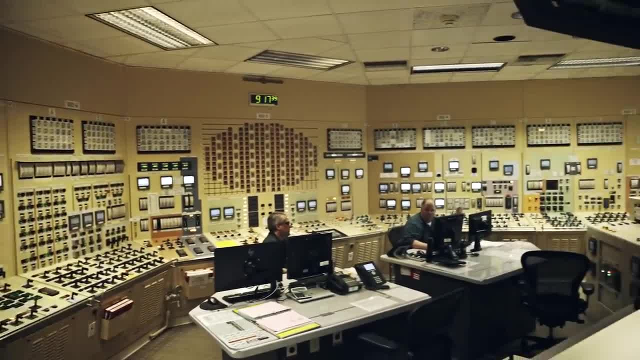 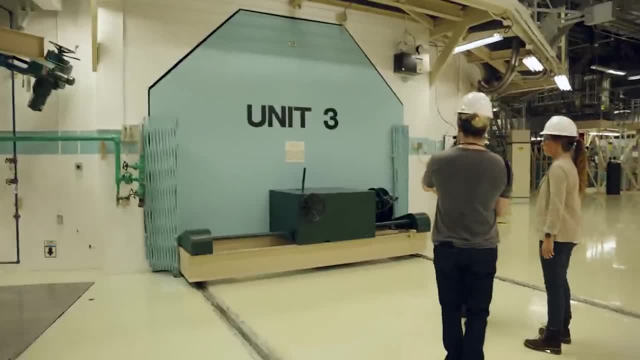 What was as clear to me, though, as the commitment to security and safety, was the fact that everyone at Dresden, from security to engineering, to public relations, were just people, and big old nerds at that. The first thing you see as you enter the facility is a Star Wars. 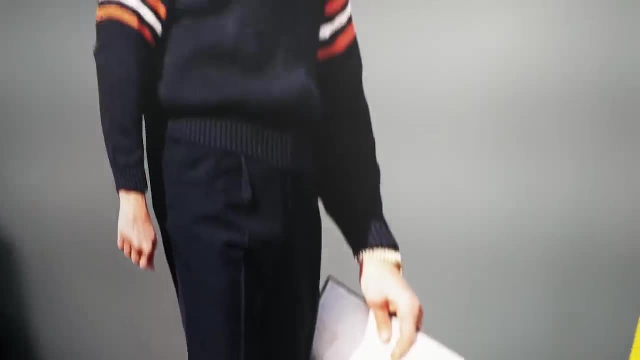 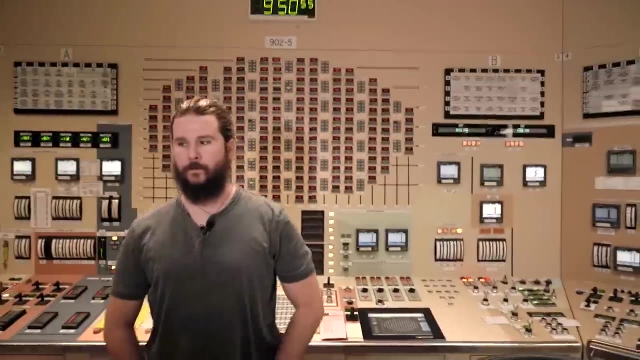 style statement about precision and safety. A poster of famed football coach Mike Ditka reminded plant personnel about radiation dosage. We cracked jokes and traded stories about Chernobyl tours which one of our tour leaders had also been on. If the public has any kind of perception, 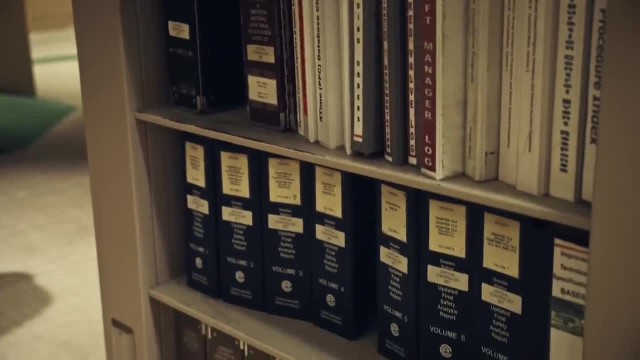 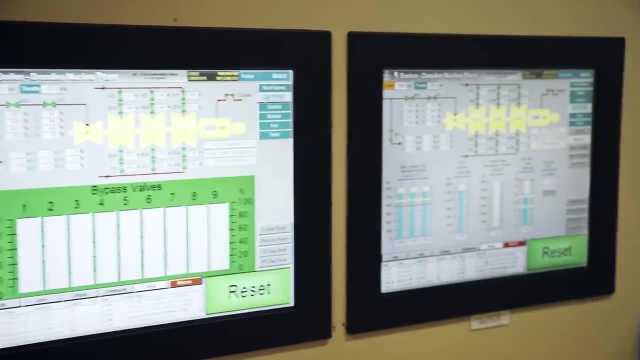 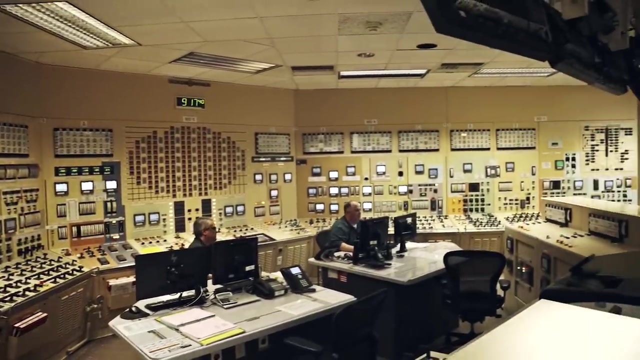 about what goes on inside a nuclear power plant and who works there. it seems negative, no doubt tinged by what they think about nuclear generally. But I can tell you that if you're friends with any engineers, if you like me at all, I think you'd be pleasantly surprised by the people who commit themselves to sustaining. 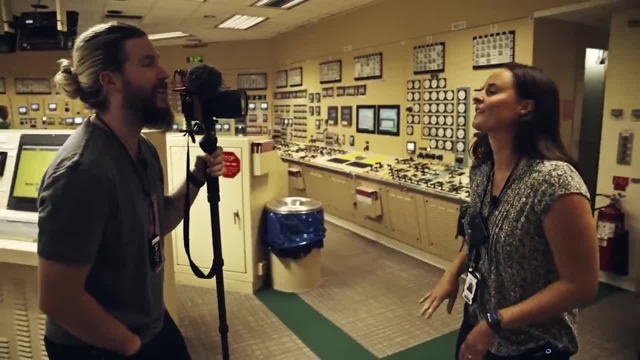 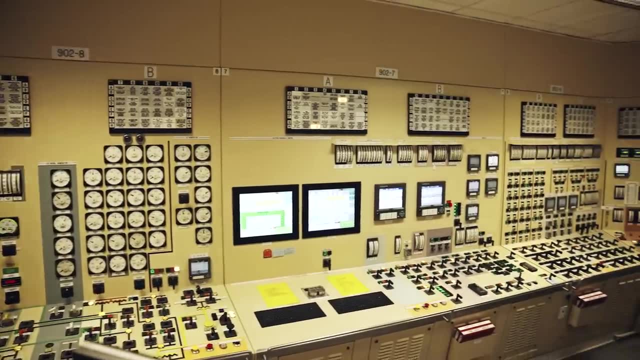 nuclear reactions. Dresden, even half-jokingly, offered me a job and that's now my backup plan. My first stop was the nerve center of any working nuclear plant, the control room. So this is the main control room for Dresden. On this side we have unit two. 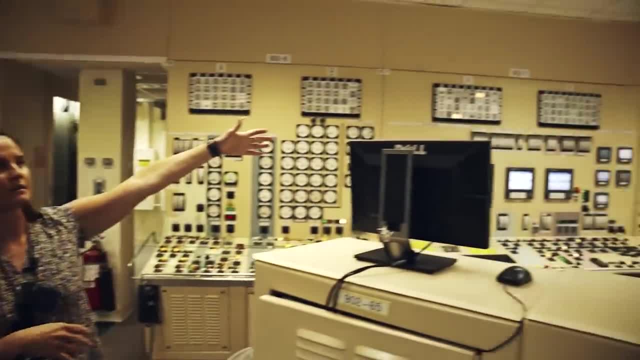 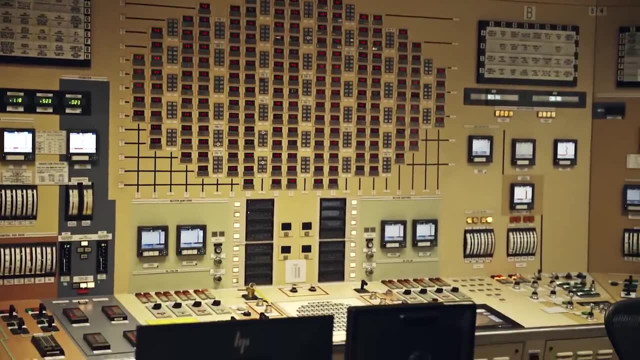 on this side we have unit three. So if you look in the center of this, it says 9025, you got the big general electric and the clock at the top. If you look at the big football-shaped item in the middle with the red, a lot of red 48s on it. 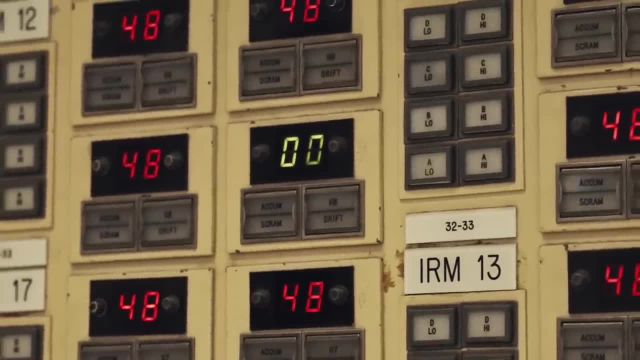 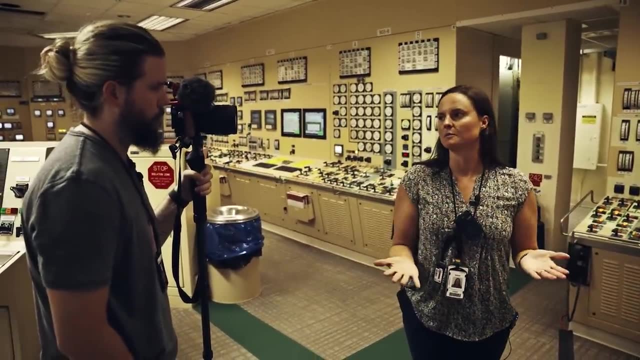 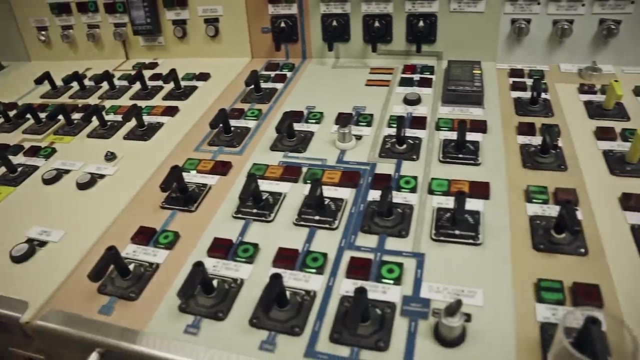 that's actually the control rod positions for the reactor core, So you can see all the control rods. The 9025 panel also has all of our big picture systems for the reactor. You'll also see on all the panels that there are color coding- human factors. The different colors designate the. 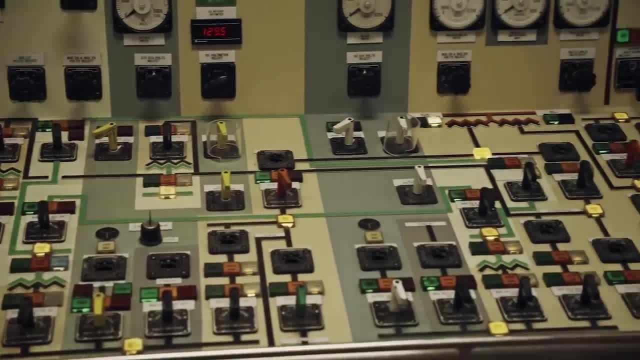 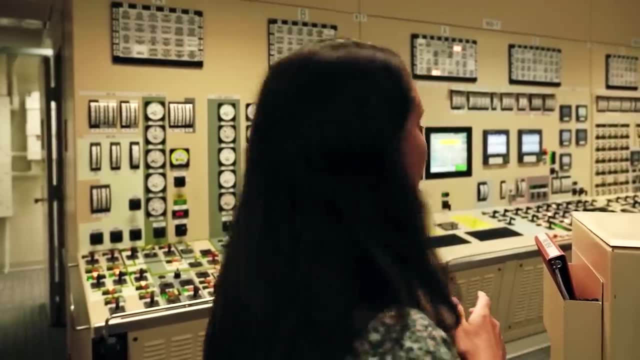 different systems. So that allows the operators to know exactly where they're going, making sure they're on the right system, and be able to diagnose any items that come up on that panel. Behind me we have the 9028 panel. That's actually our power distribution panel. So all of our 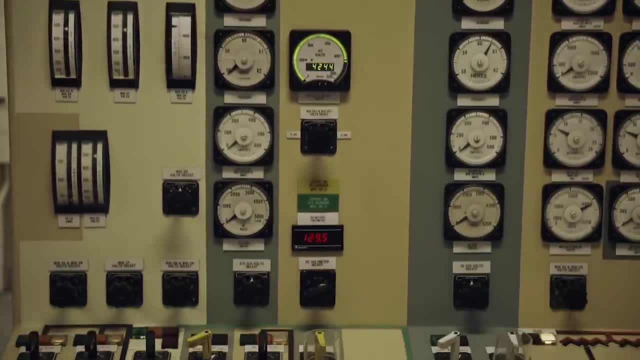 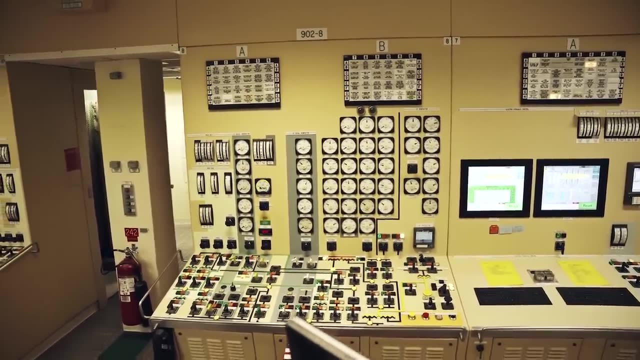 different buses, that power equipment and our plant are located on that panel, And then also our voltage regulator, which is how we control the power that goes out on the grid Here at the Dresden Nuclear Generating Station. like any other modern nuclear power plant, safety is the top. 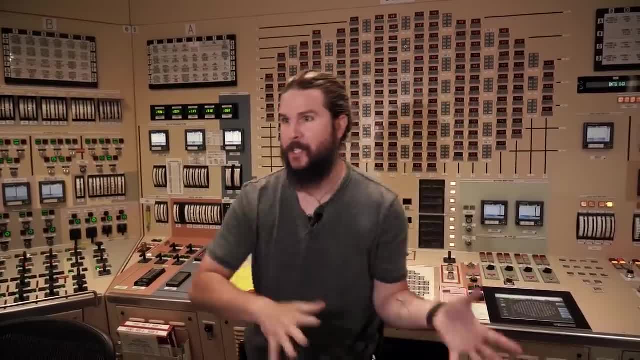 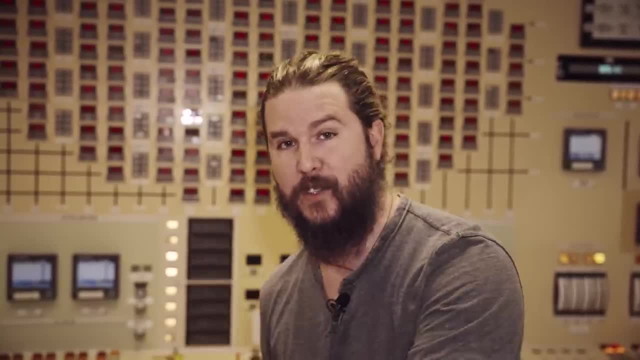 priority Now. I know you see a lot of buttons, switches, knobs, valves. It can all look complicated, but a lot of design has gone into making this as safe as possible, as operable as possible After accidents like Three Mile Island. 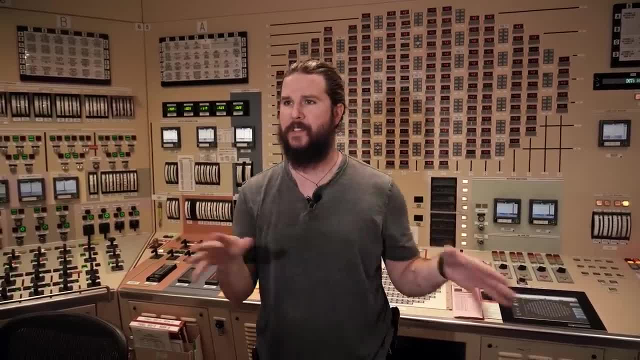 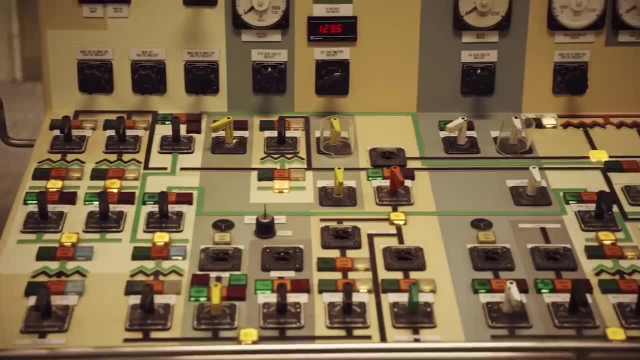 a lot of thinking went in exactly how to make all of these systems immediately understandable, recognizable. Before that, it was just blinking lights. You have color coded panels that tell you exactly what you're working on, exactly what you need to adjust or not. You have mock-ups of the 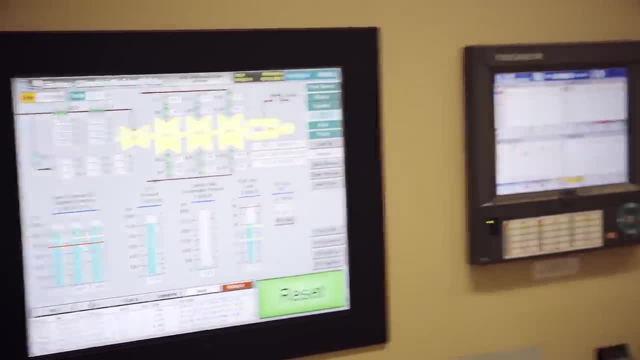 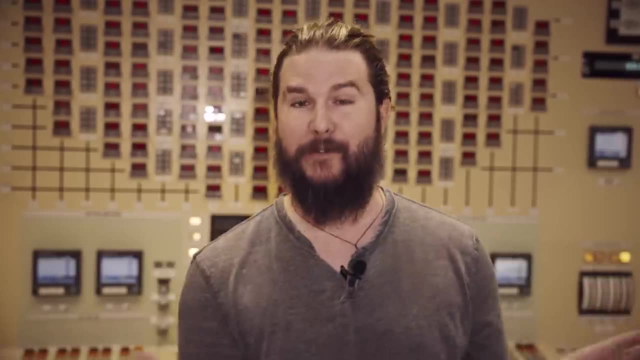 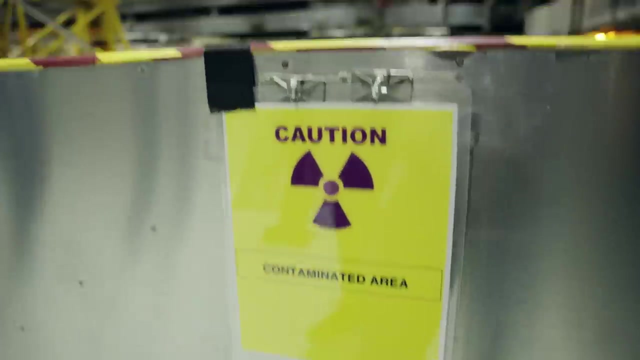 actual system, Whether it be the turbines or the boiling water reactor itself. it tells you what valve goes where, what needs attention and what does not. Safety, again, is the top priority. From the control room we headed to the spent fuel pools at Dresden, where highly radioactive. 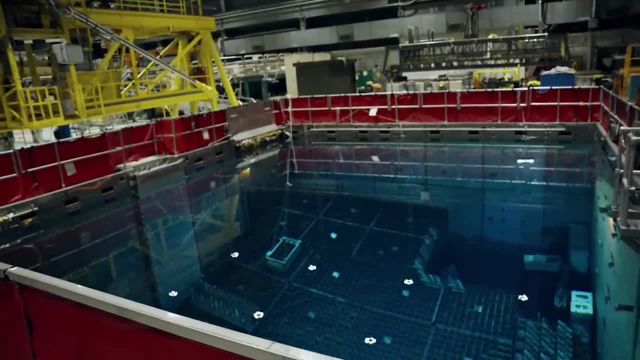 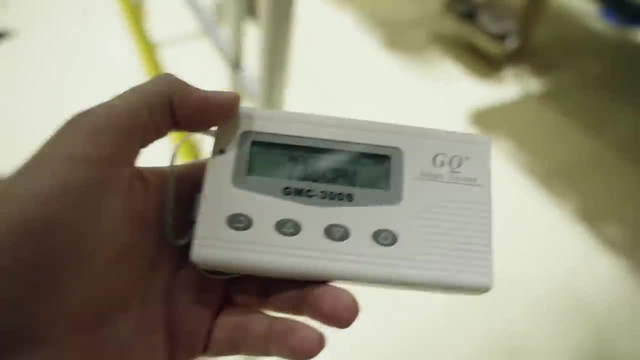 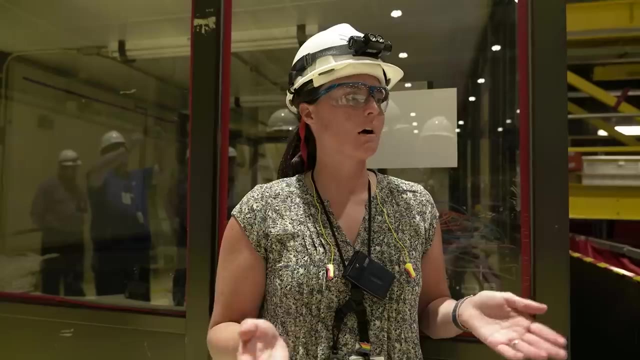 fuel rods cool and decay to safe levels after years of geometrically determined placement throughout reactor cores. This was my first time seeing real nuclear waste and my first time seeing the infamous Cherenkov radiation with my own eyes. When our refueling outage comes, all of this basically gets opened up. 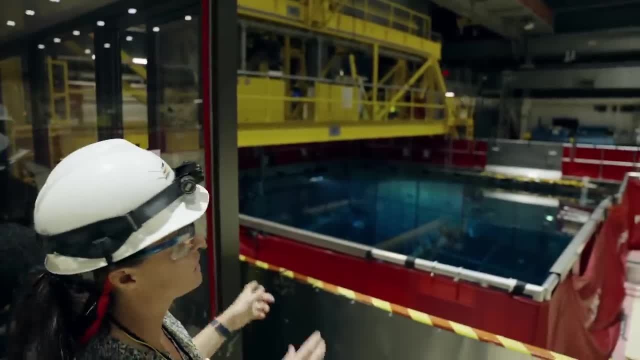 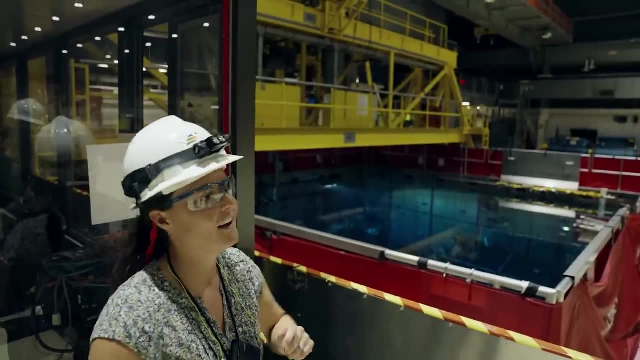 and it all is connected underwater. We use this bridge to pick up fuel bundles: take it from the reactor, put one in the spent fuel pool. take one from the spent fuel pool, put one back in the reactor. It's not that simple, though. There's about a thousand moves that have to occur to get. 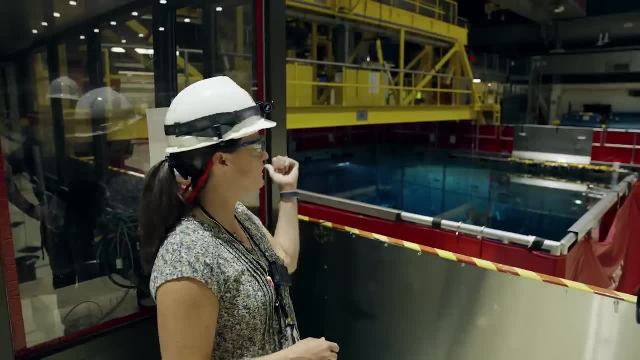 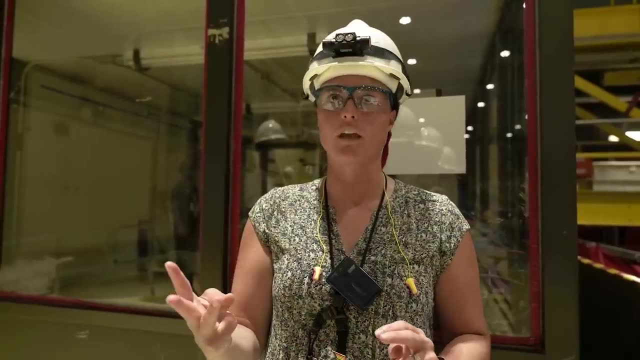 everything reshuffled and into the right locations. There is always a senior reactor operator on the bridge controlling all the fuel moves during an outage. so there's actually three verifications that occur: The performer, a reactor services individual and a senior reactor operator make 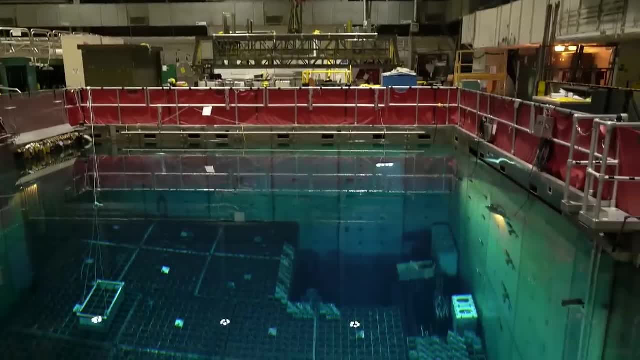 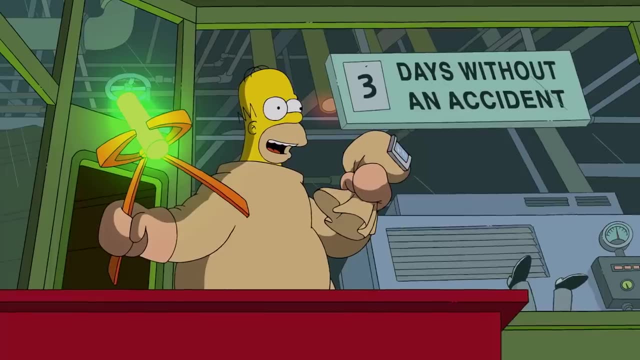 sure that all the fuel is going to where it's supposed to be going. As a quick aside, radioactive stuff- nuclear waste- doesn't glow, Not by itself. The idea that nuclear waste glows green, like in The Simpsons or something, is probably traceable to one of the 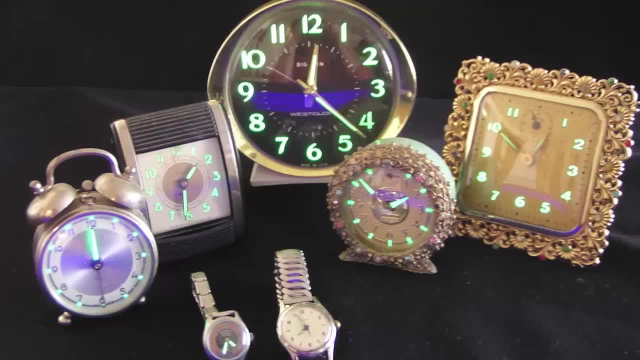 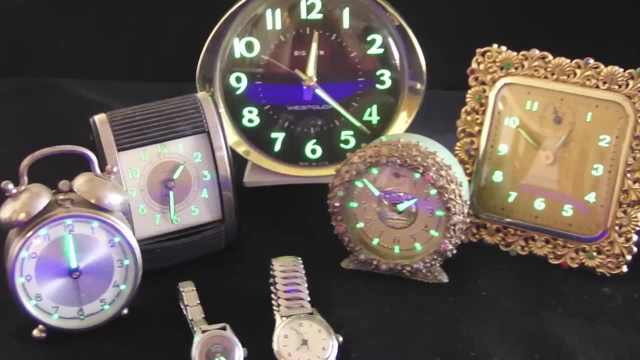 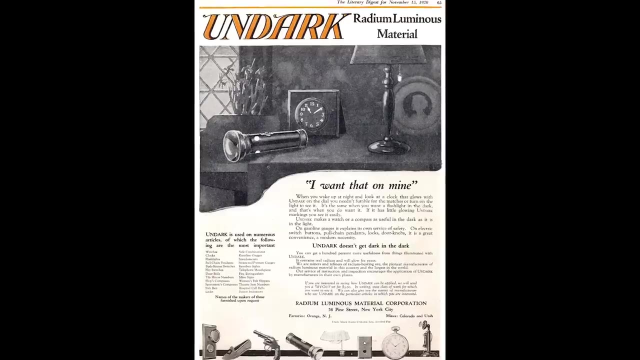 first popular consumer applications of radiation Undark, a luminous paint containing radium. The highly radioactive element would energize the zinc sulfide in the paint, which would in turn fluoresce a soon-to-be-characteristic green. Undark would light watches, gun sights and more at the start of the 20th century – that is. 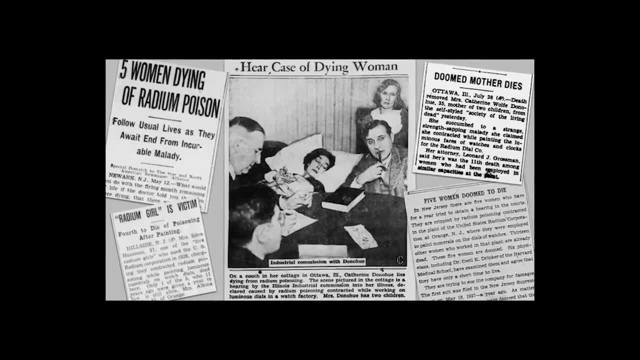 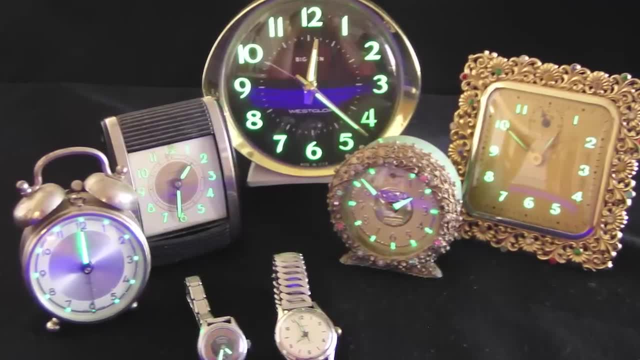 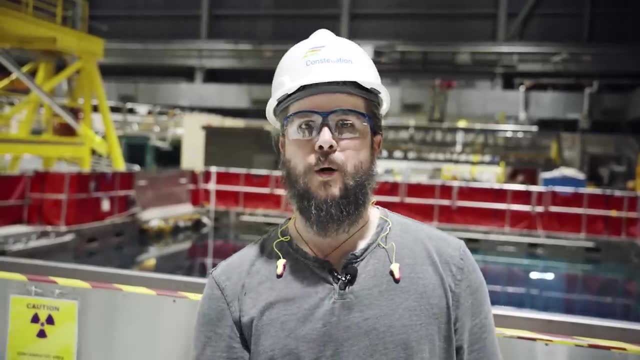 before. the tragedy of the radium girls that worked with the compound became public and the use of the paint declined, The point being that radium doesn't by itself. Nuclear waste doesn't glow, Nuclear fuel doesn't glow. Behind me, probably one of the 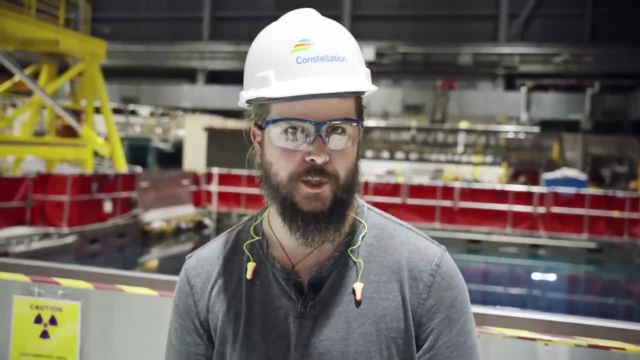 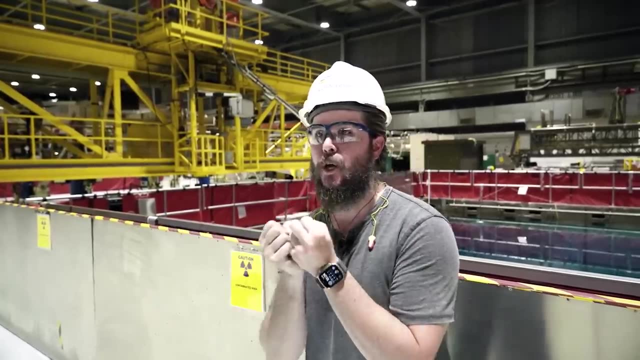 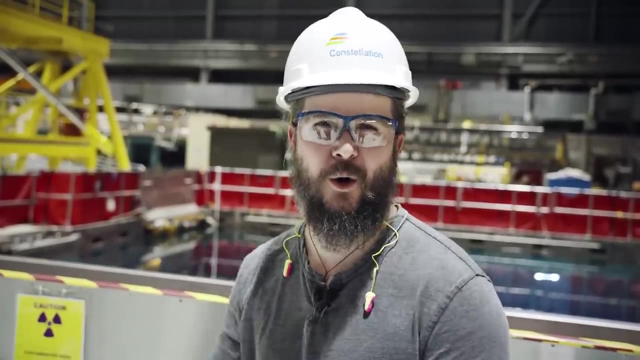 most iconic images you can find in any operating nuclear power plant: The spent fuel pool. Behind me you see fuel rods producing that characteristic blue glow, that Cherenkov radiation. You probably have an idea in your head that nuclear waste is some goo thrown in a barrel and then discarded. 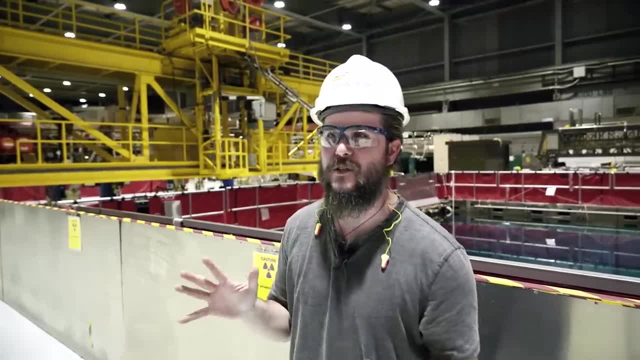 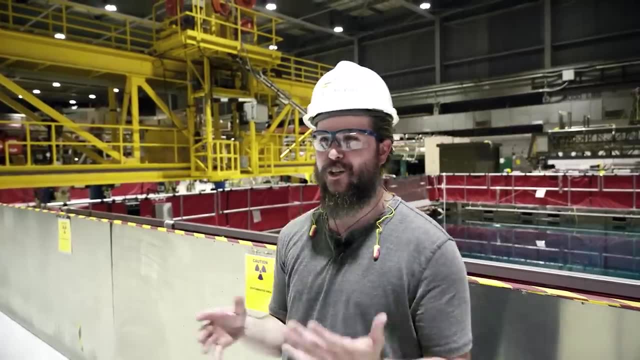 forever and never thought about again. Nay, dear viewer, I say that it is an intensely clean and organized operation. Behind me you see how everything is cordoned off here. They won't let me get any closer than this because they're worried that something like my hair tie will fall. 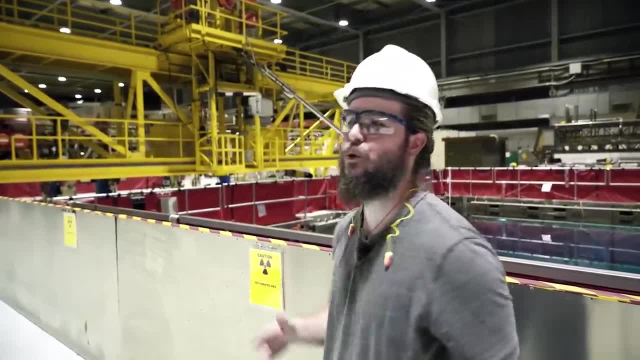 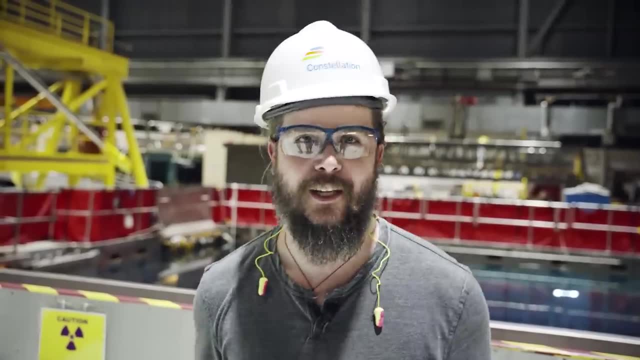 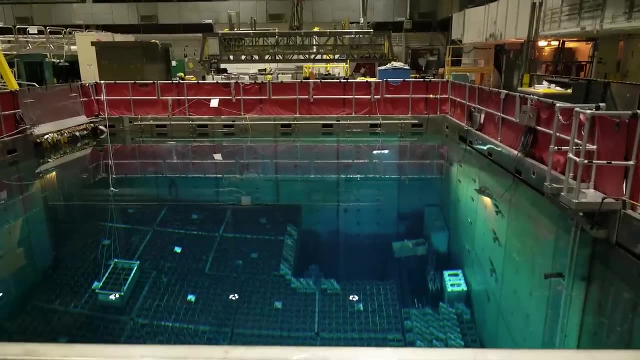 into the fuel pool and that could contaminate the fuel. It could damage something. It could make its way into the reactor during refueling. This water is cleaner than I am and it's nuclear waste: Innumerable near-light-speed particles creating sonic booms of light in water- Cherenkov radiation. 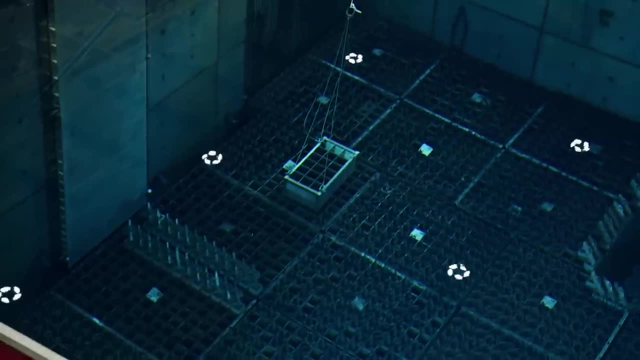 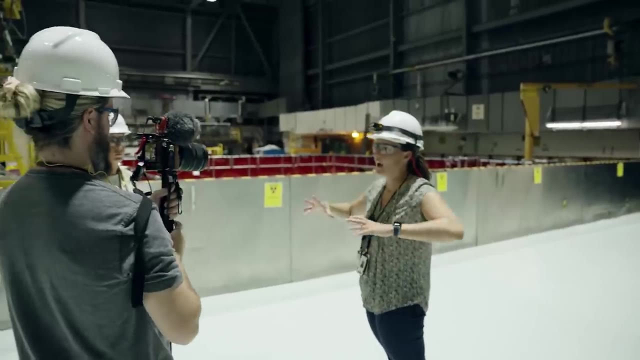 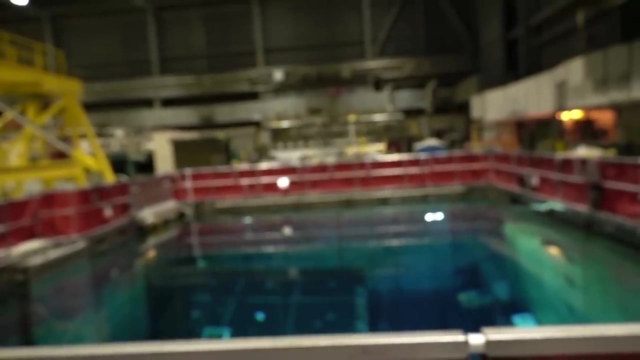 is awesome, but it's also not nuclear material glowing. Clearing up this misconception helps you see nuclear waste for what it really is: Pretty uneventful. I should also note here that, though our personal dissimilators that you're seeing in this video were showing increased radiation rates. 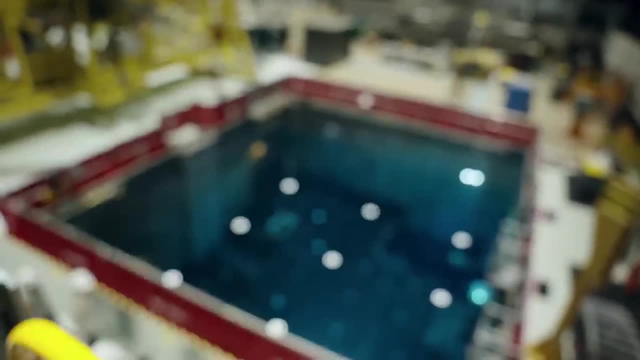 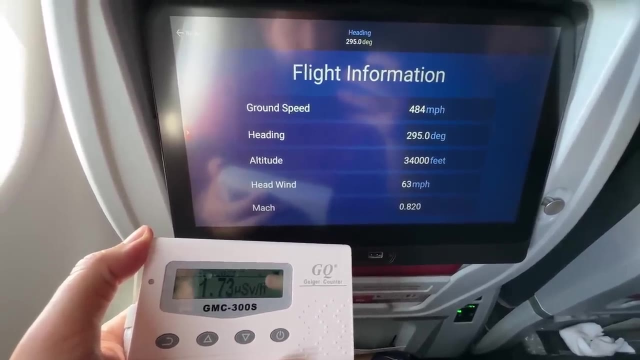 near the spent fuel, which makes sense. it was only about the amount of radiation that was released at the same rate as you'd get at cruising altitude in an airplane, which is much lower than I'd guess the average person would think. After the fuel pool, it was time to see where any 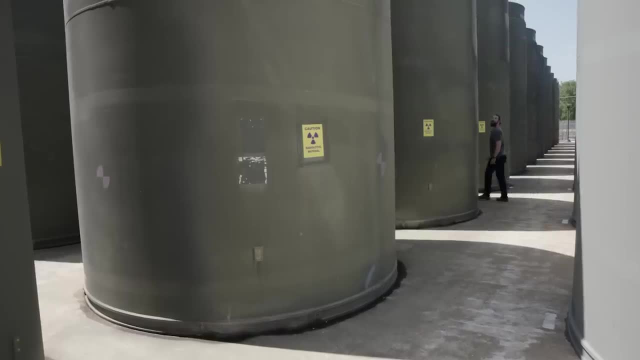 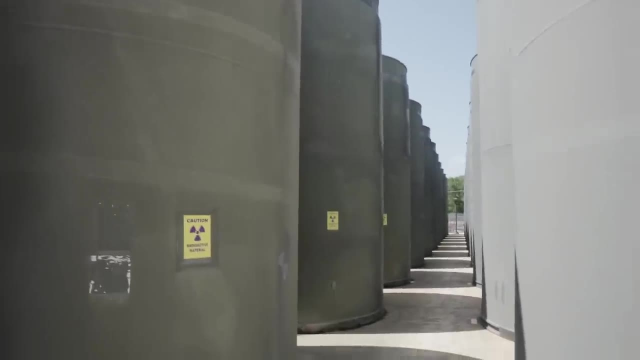 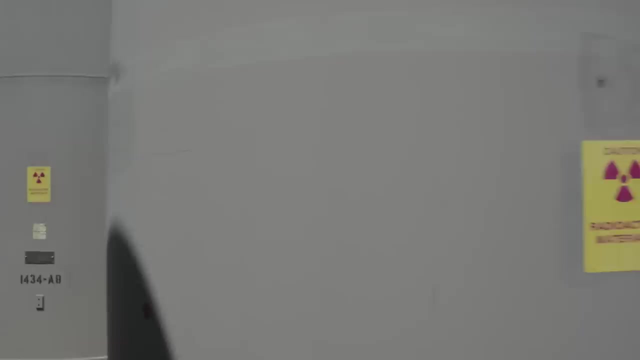 operational nuclear plant stores the majority of their waste Dry casks. When you think about nuclear waste, don't imagine glowing barrels, Don't imagine green goo. Imagine these Towering plane- and missile-strike-resistant monoliths of steel and concrete housing waste that has 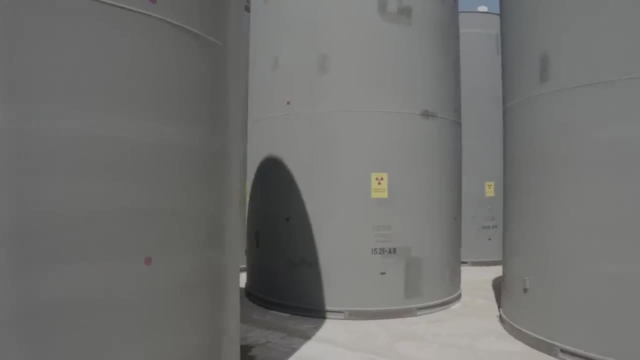 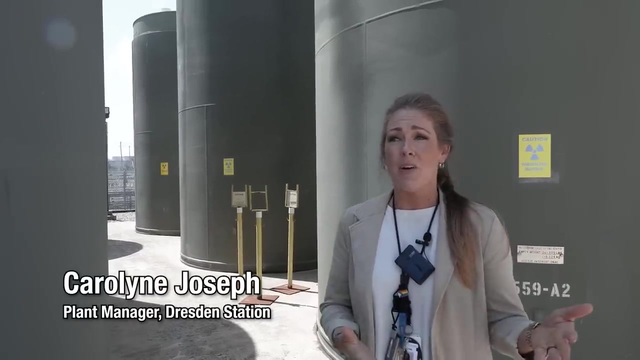 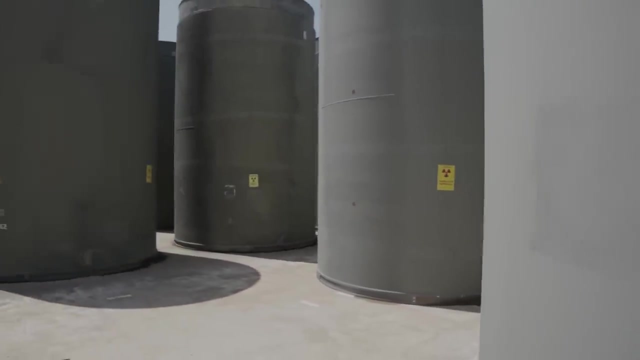 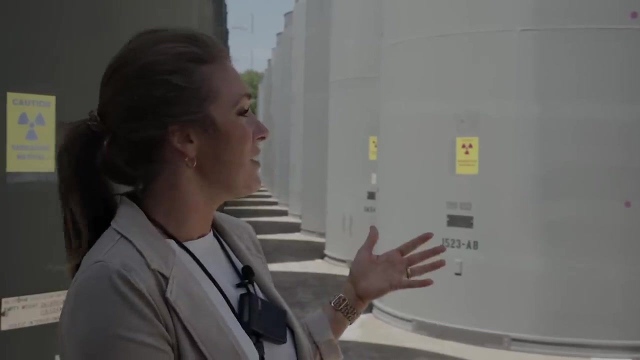 been melted down and frozen in stone. This is our west pad for our independent spent fuel storage installation. This pad on it has about 71 dry cask assemblies. This one is for units two and three. What we have here, these casks are about 16 feet tall. They hold 68 fuel bundles apiece. So inside of these casks, 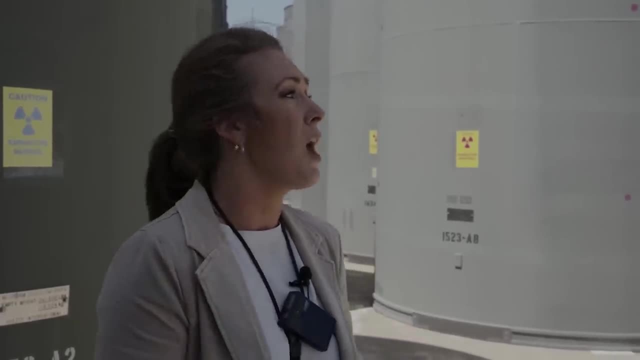 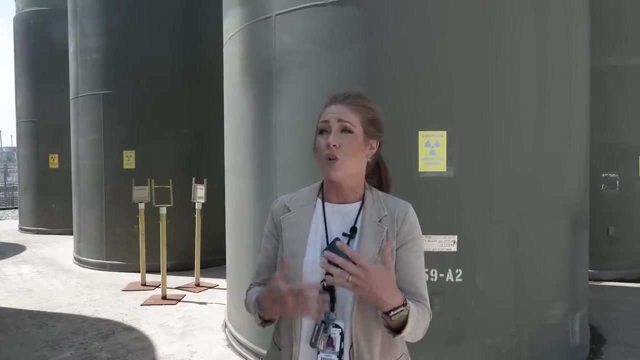 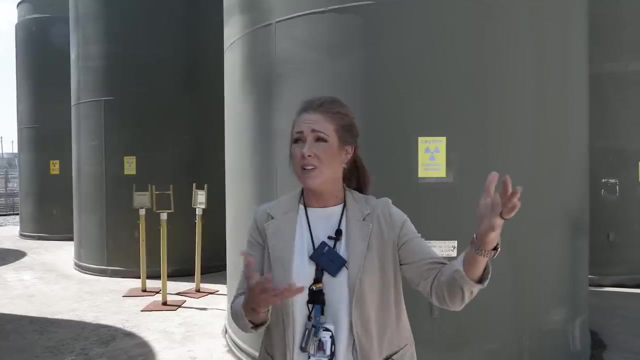 we have our MPC that actually holds the fuel bundles. We completely dry that out. We put helium inside of it to de-inert it so that there's no oxidation going on Inside of those fuel assemblies. we put it inside of these concrete canisters which are a little under three feet. 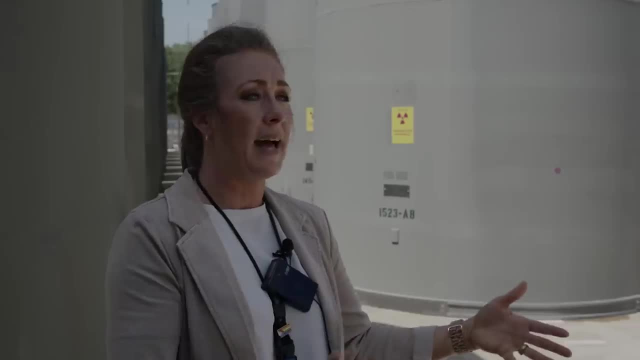 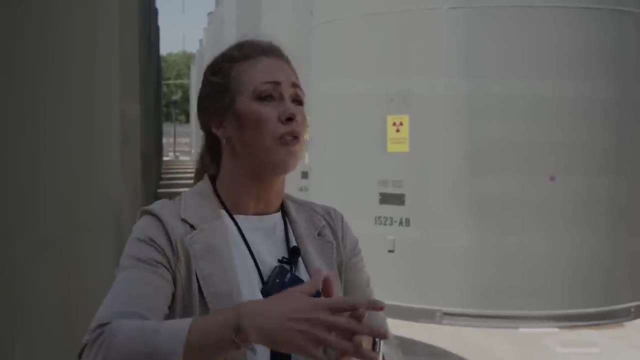 thick And then we put them out on this pad. These pads are designed to hold all of the nuclear fuel for that specific duration of the license. So unit one pad holds all of the fuel for unit one. It still has room on it for additional casks. This pad has 13 additional casks. This pad has 13 additional. 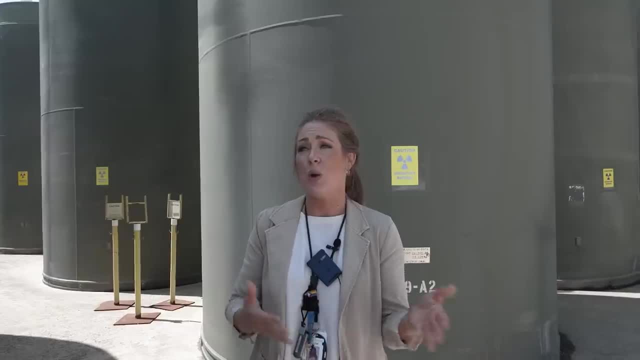 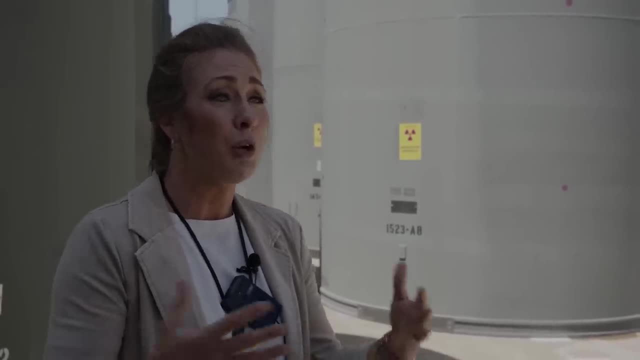 spots available to hold the spent fuel from unit two and unit three for the duration of that license. So with the over 100 nuclear reactors that have been operating since the 70s, if you were to put all the nuclear waste in one location, it would all fit on one football field. 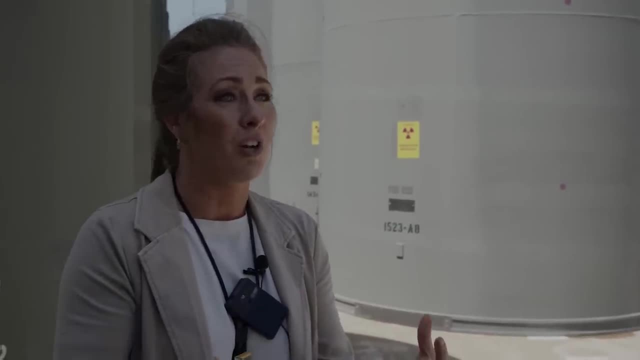 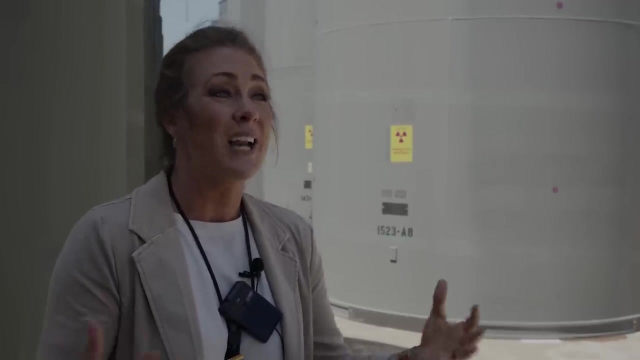 You know. so for you and I, the amount of waste that we would generate, related to what we would consume in nuclear power generation, is equivalent to one Coke can, So comparatively not a lot of waste, especially when you look at some of the other power generation industries. 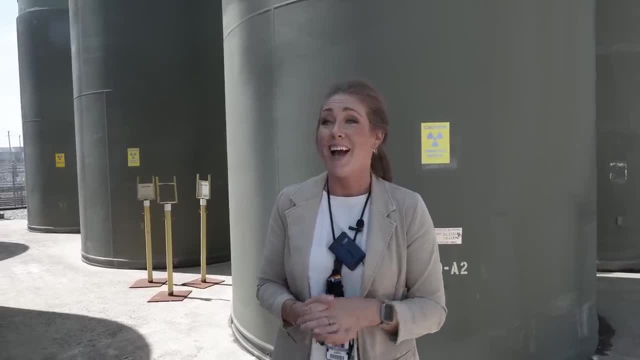 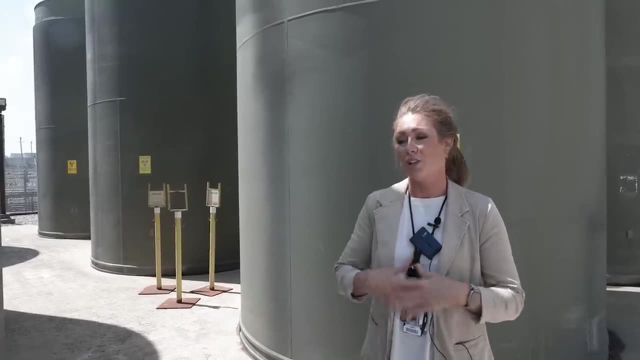 Would you be worried about living next to any of these casks? I would not. I would put it in my backyard. I would go like right and hug it. They're you know they're incredibly, incredibly safe. you know low radiation emission, So I would. 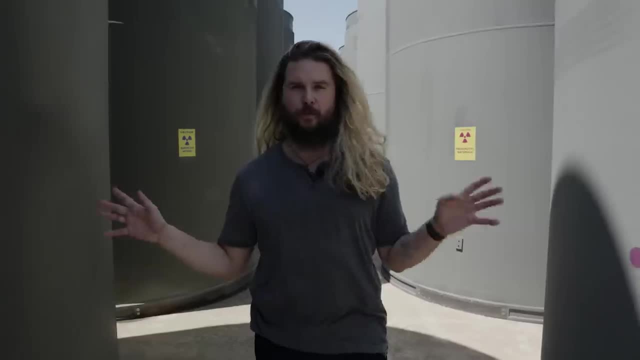 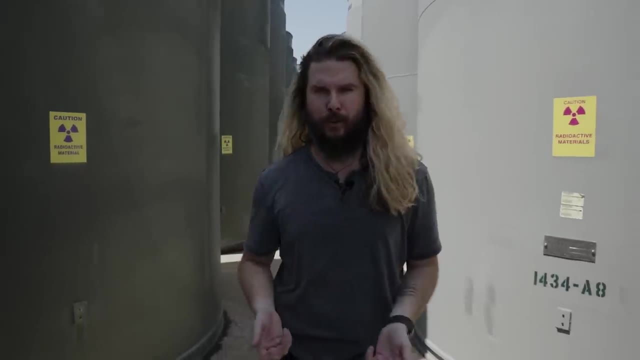 certainly have one in my backyard. This is where the rubber meets the road when it comes to nuclear waste. I know many of you have an idea in your head that it's some glowing green barrel of goo like you may have seen on The Simpsons. No, Though it is still cylindrical, nuclear waste is stored. 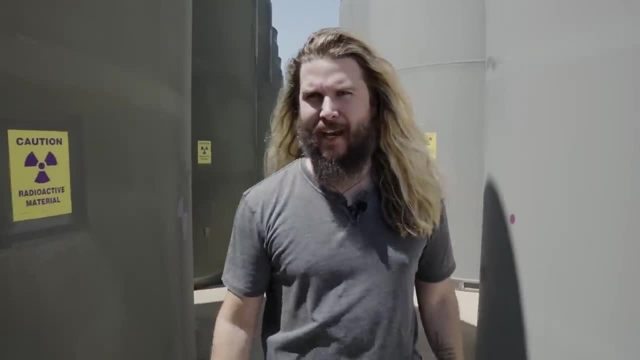 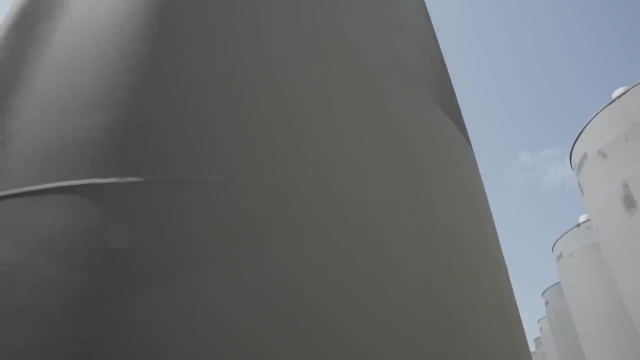 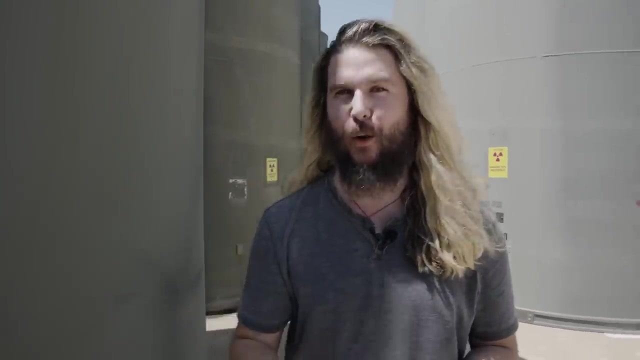 in rock form in these enormous dry casks. Here they can stay for an entire lifetime of a plant, mostly inert, decaying down to the point of harmlessness. There's nothing to leak here. In fact, there hasn't been a single recorded case of nuclear material leaking out of any of these. 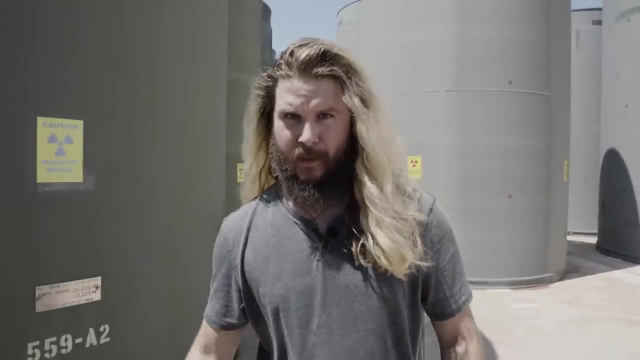 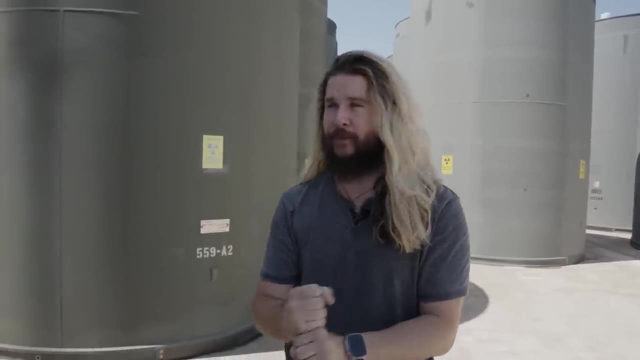 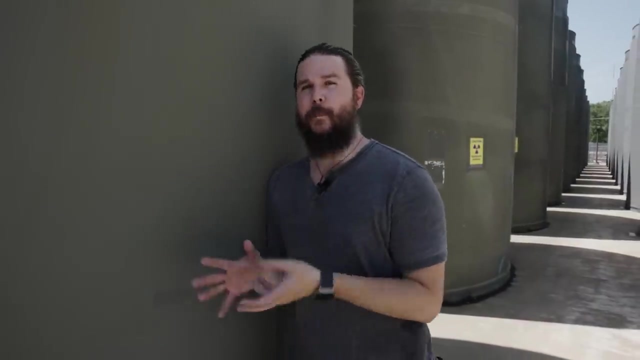 in the United States anywhere ever. When you're talking about robust safety, when you're talking about managing nuclear waste in the correct, safe way, it doesn't get much more straightforward or safe than this. And while we're talking about nuclear waste, think about where nuclear waste is, What 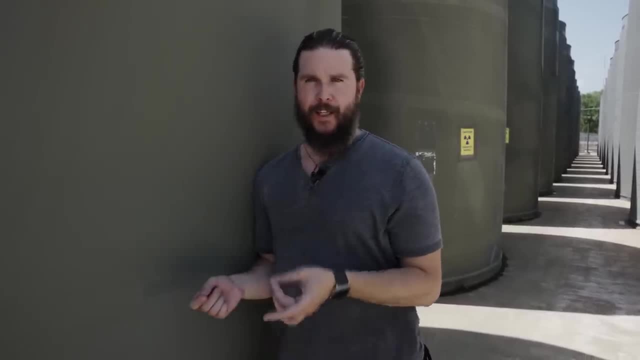 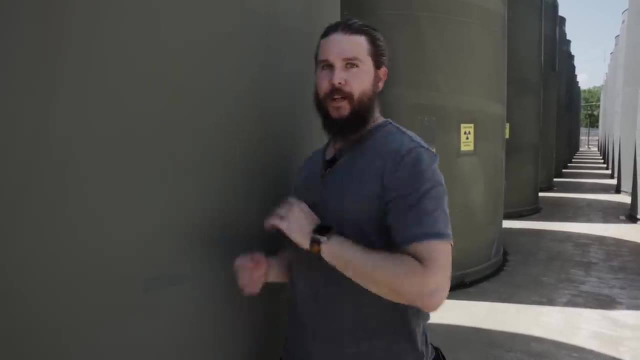 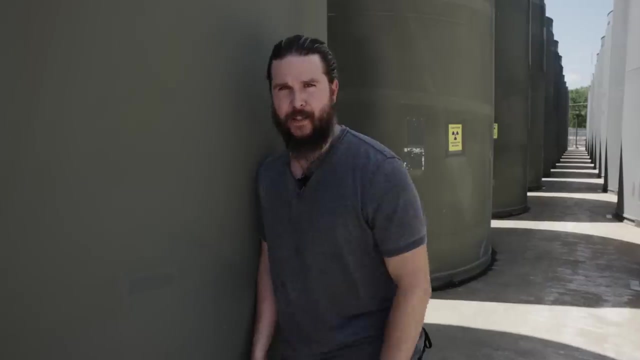 Constellation likes to say is that they can account for every neutron. Can you say that for any other industry? about anything? Probably not. Where is the nuclear waste at a nuclear power plant? It's in the fuel pool, It's right here. Where is the waste from a fossil fuel plant? 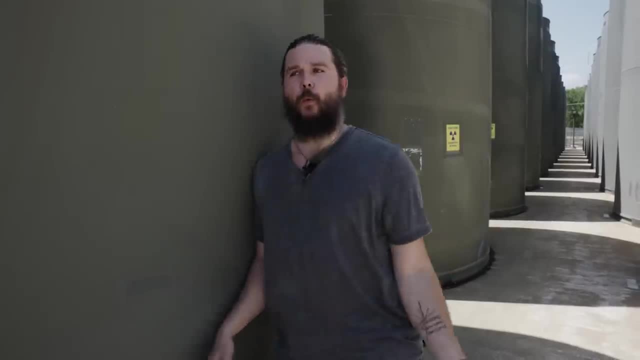 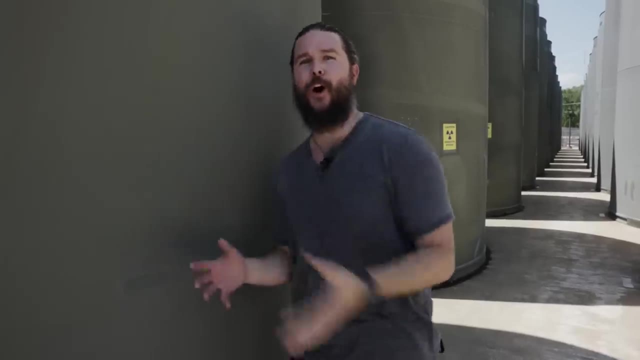 It's in there, It's in the air, It's in the ground, It's in the water. What about the mercury? It stays toxic forever. Do you know what doesn't stay toxic forever? Decaying nuclear material. When we talk about pollution, we need to have a fact-based conversation about this. Nuclear does produce some. 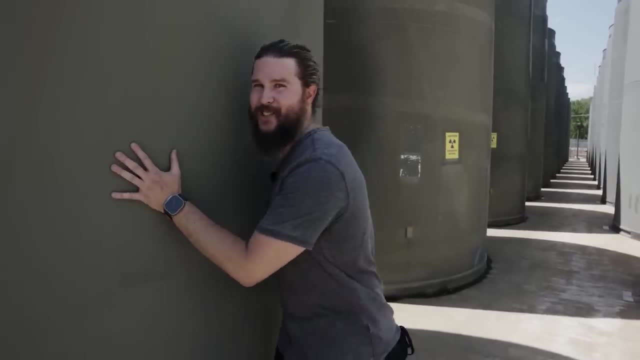 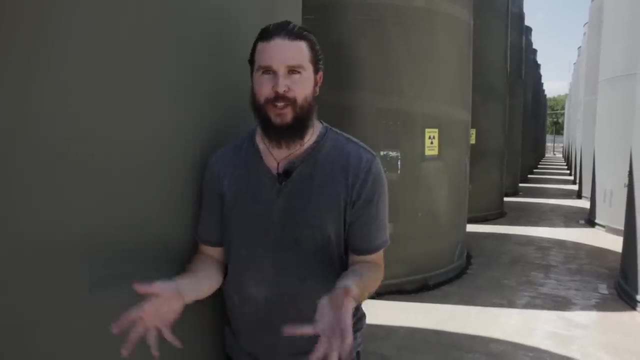 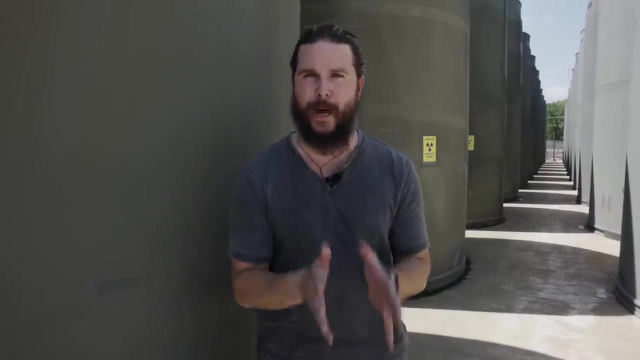 pollution- It's all right here- accounted for in casks that could repel, basically Superman. Where is all the pollution for the fuel that we are using for the last 100 years? It's in your lungs. It's making your kids' IQs go down. We have to talk more sensibly about pollution. if we're all 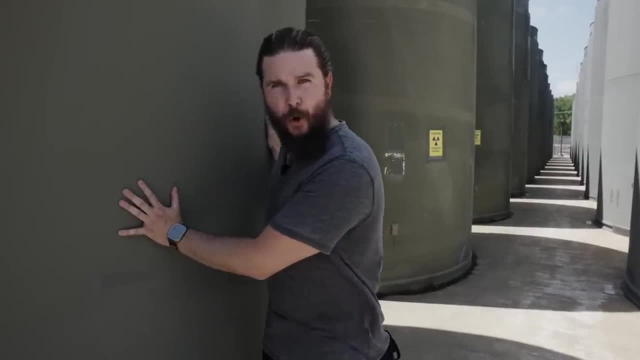 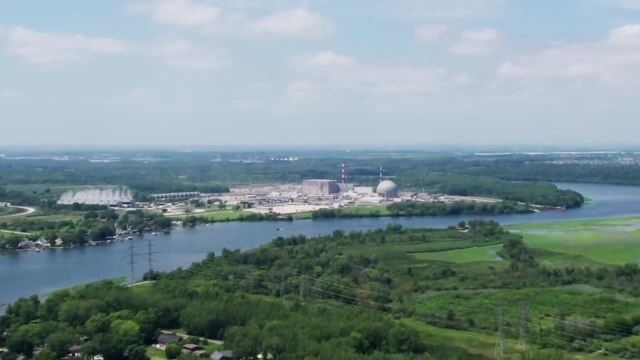 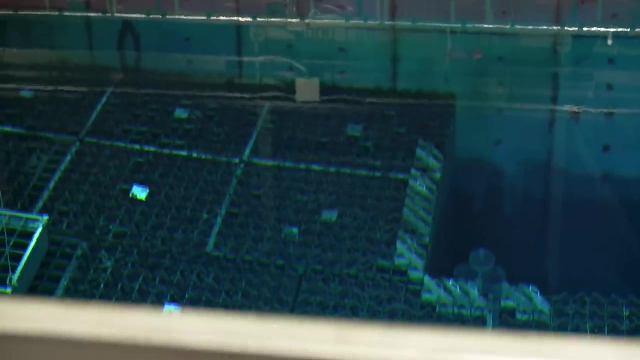 going to get more sensible about how to deal with climate change and our growing energy dependencies. It is not an exaggeration to say that nuclear waste contained within nearly indestructible casks and piled in pools of water cleaner than the water you drink may be the safest waste there is. 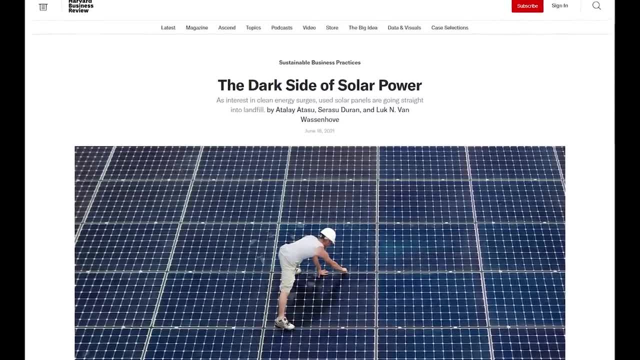 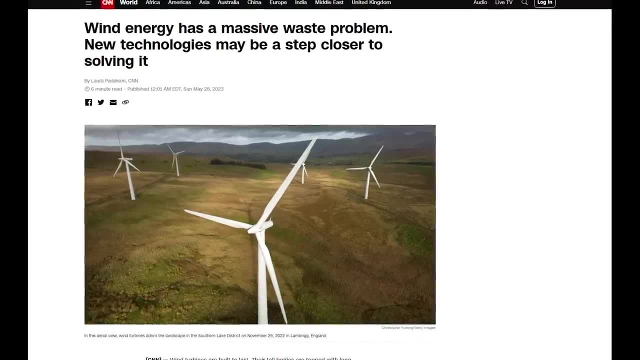 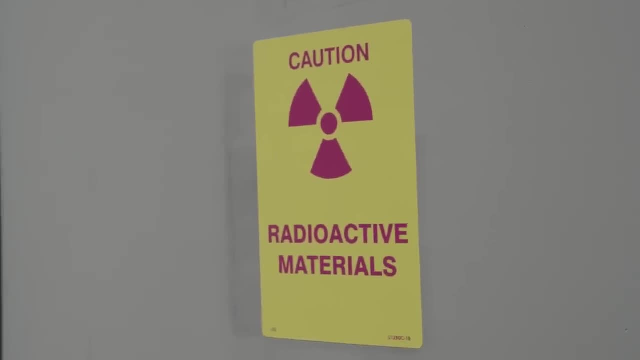 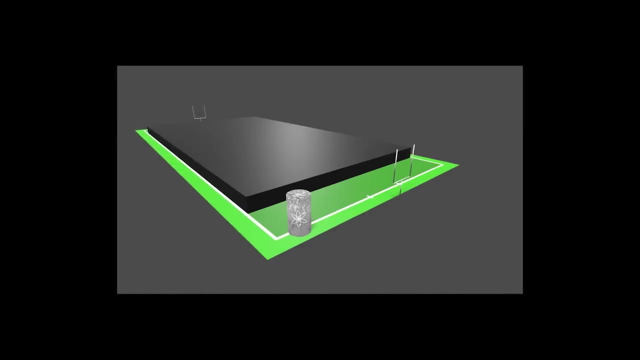 Use solar panels containing heavy metals live forever and stay toxic. All of the waste produced in a nuclear power plant's lifetime, in comparison, can live on-site, getting less dangerous as it does. so All of the nuclear waste in the world could now easily be. buried in a single deep earth repository, thousands of meters below any water table or geologically active area. If we had the political and public will to do so, I wouldn't be able to make a point like this. if it weren't true. No, literally, There are armed. 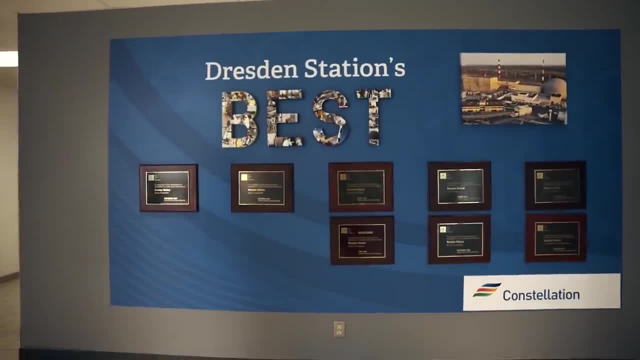 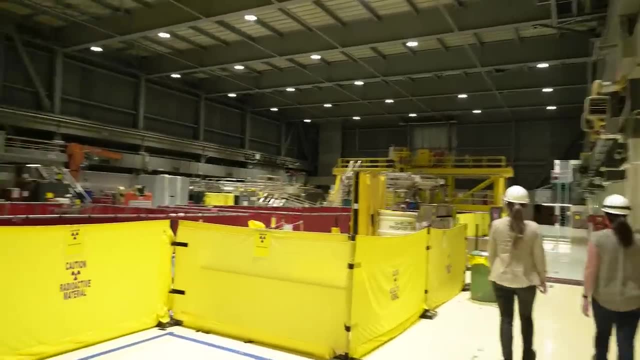 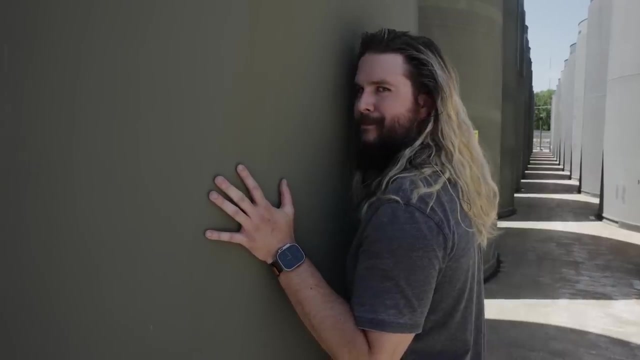 guards and a public relations team on the other side of the camera. right now, The relative safety of nuclear waste is both theoretically and practically proven, And if you still don't believe me about that…. My tour of the Dresden Generating Station was my first. 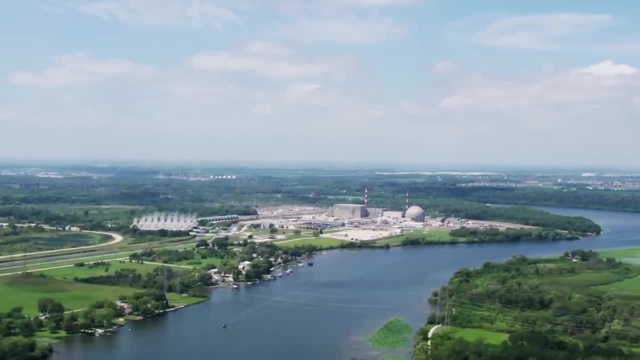 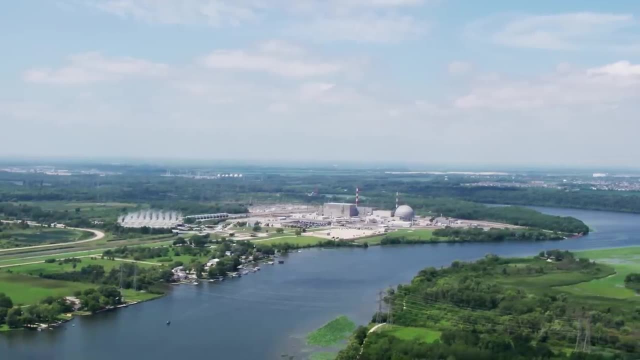 and most important visit of the power plant that hadn't exploded. And it's now even more clear to me that nuclear disasters, like the many I have featured on this channel, are the exception, not the rule. Modern nuclear technology is extremely robust, redundant and safe. It's. 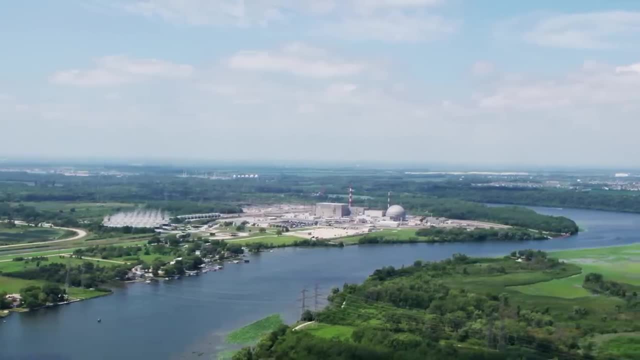 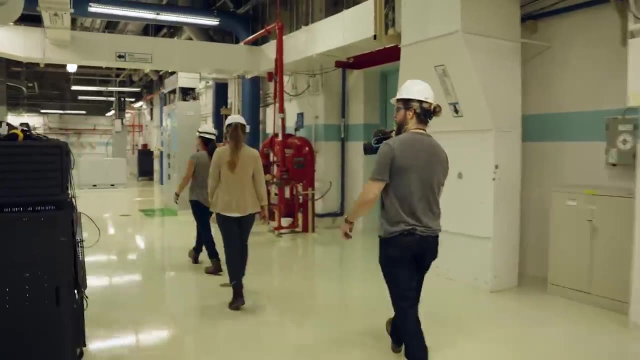 only when human error combines with poor and or flawed design that you get a Chernobyl, Fukushima or Three Mile Island. I wouldn't say that nuclear power will solve all our energy problems And it can't be the only solution. I would say that it's more than a dream. It's a dream. I'm not sure if it's a dream, but it's an answer. But if you want to get to know it, you have to go and see it, And if you want to get it, be sure to do so. It's a dream. It's a dream When you think about it. you're not going to forget it. 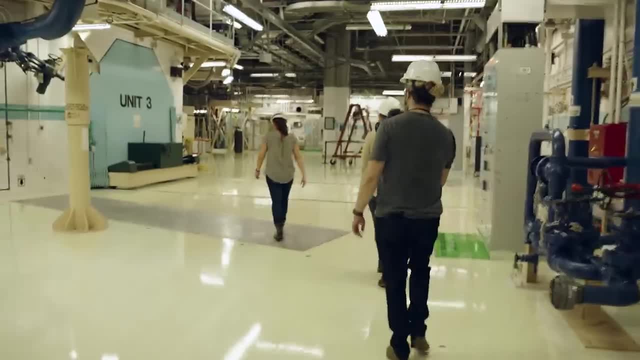 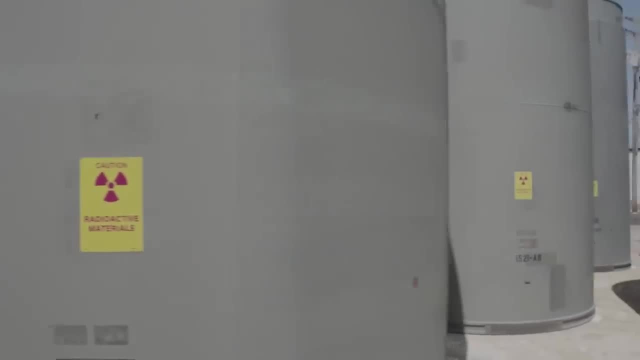 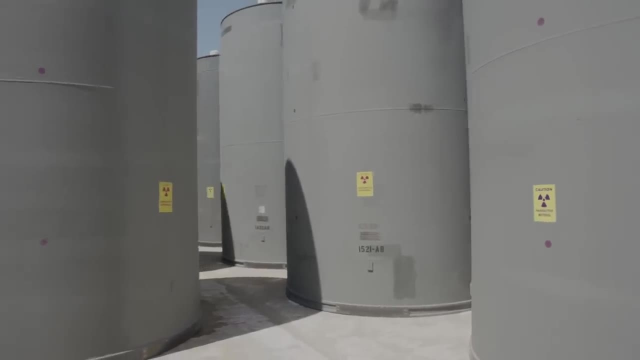 it can't be the only solution to climate change And it has its own economic and political challenges, though many of those are easier than they seem. But I will say that opposition to nuclear power that relies on arguments about the safety of nuclear waste specifically, is misinformed at best. 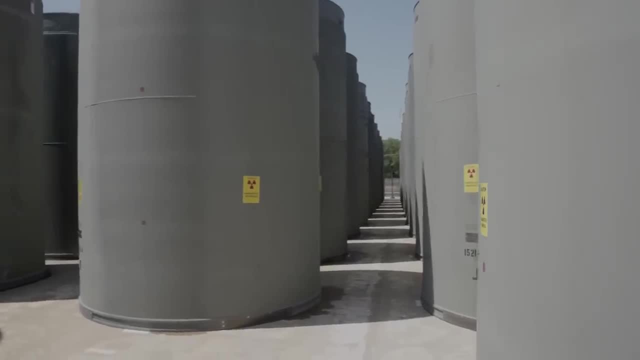 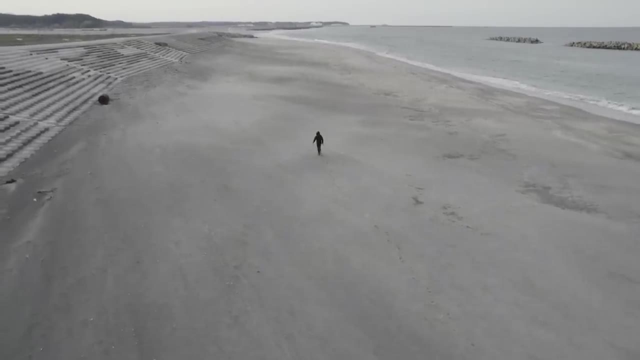 and monetarily or emotionally motivated at worst. I walk through exclusion zones, eat Fukushima sushi and literally kiss nuclear waste containers, not because of some weird obsession or fetish, though I know some of you probably think that at this point- and yes, 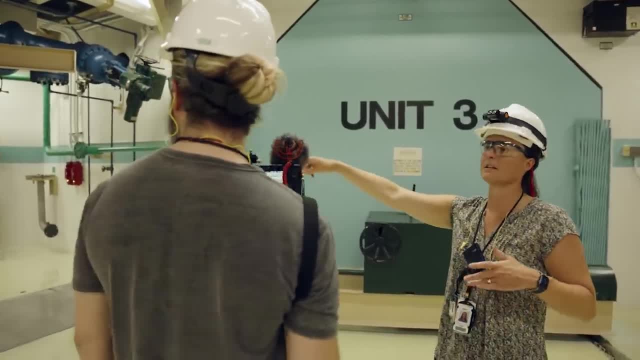 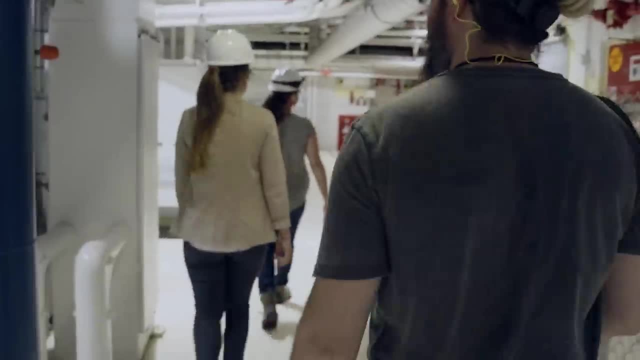 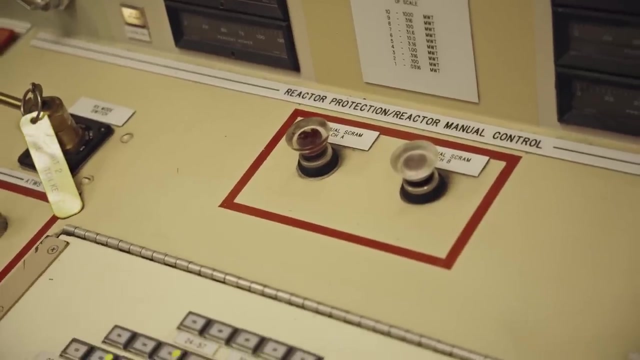 I did ask Dresden if I could swim in the nuclear fuel pool. I do all of this to prove a point, And that point is this: The world looks different when you understand it, And nuclear power and waste, when you understand it, looks less dangerous and more promising than ever. Until next time.